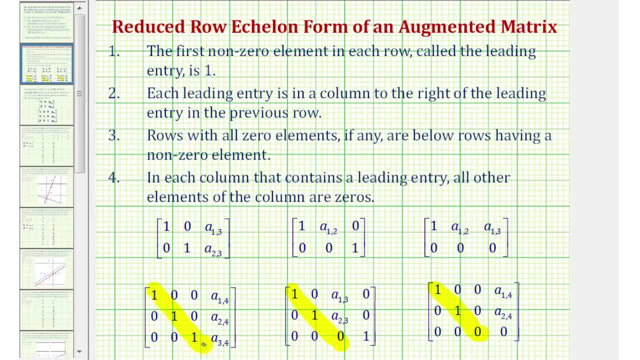 where? notice: if the main diagonal only contains one, we have one solution. If the main diagonal contains a zero, we have either no solution in this case here, or infinite solutions in this case here. if we have a row of zeros, We'll transform the. 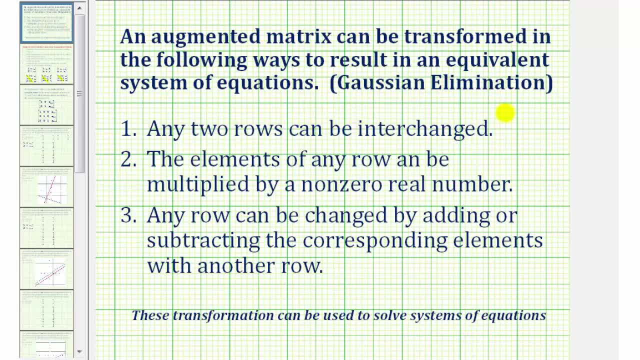 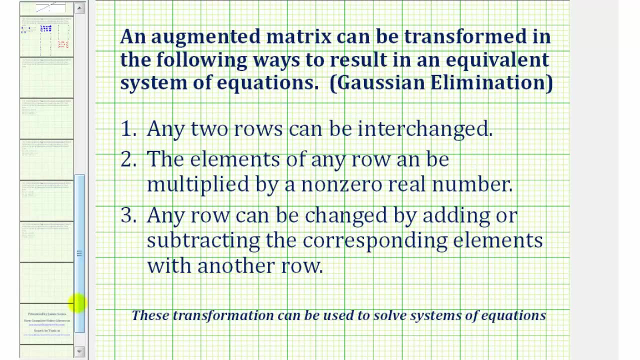 matrix into this form: using Gaussian elimination, which allows any two rows to be interchanged, The elements of any row can be multiplied by a nonzero real number, and any row can be changed by adding or subtracting the corresponding elements with another row, So this can be a fairly involved process. 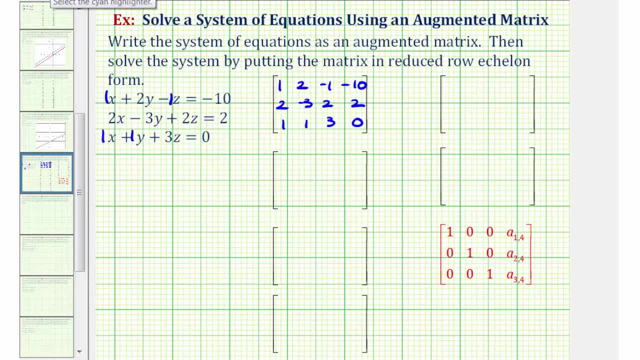 so let's start by focusing on obtaining a zero in row two, column one, and row three, column one. So if we focus on just row one and row two, if we replace row two with negative, two times row one plus row two. 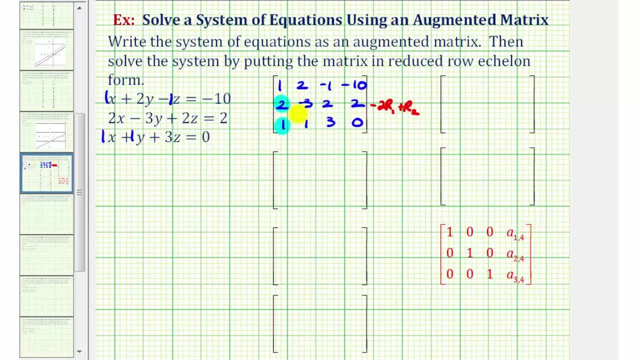 that would give us a zero in this position here And now. if we look at row three and focus on row two, notice: if we replace row three with negative two times row three, that would give us a negative two here. and if we add this to row two, 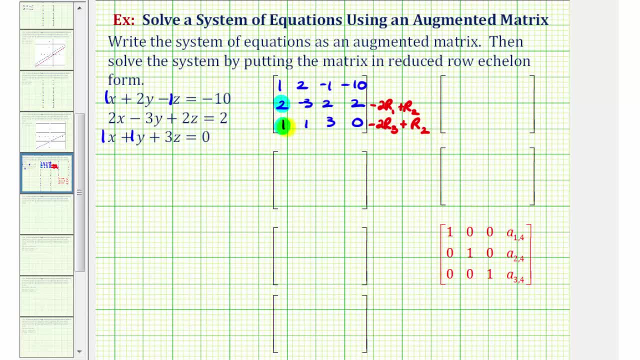 we would get a zero. Let's start by performing these two row operations. So we'll leave the first row the same for right now, And now for row two we'll have negative two times one plus two, that's zero, Negative two times. 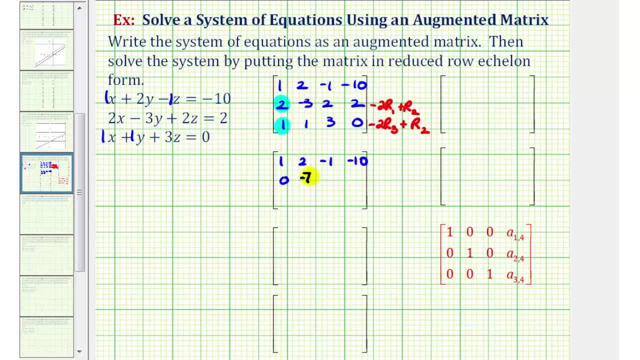 two plus negative three, that's negative seven. Negative two times negative. one plus two is four Negative two times negative. ten plus two would be twenty-two. And now for row three we have negative two times row three plus row two, So negative two times one plus two is zero. 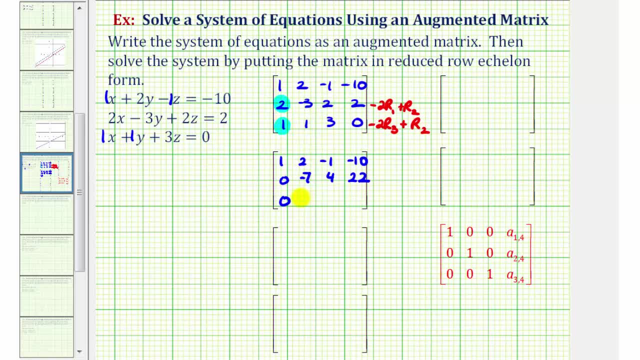 Negative two times one plus negative three is negative five. Negative two times three plus two is negative four And negative two times zero plus two is two. Now let's focus on obtaining a zero in this position and this position. Well, looking at row two and row three, 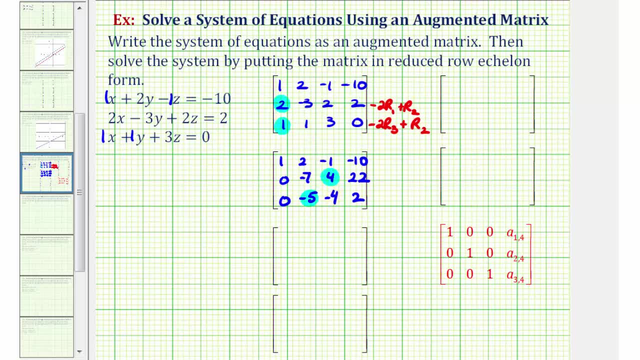 notice how the elements in column three are already opposites, which means if we replace row two with row two plus row three, we would obtain a zero in column three. We also would not lose the zero in column one. Now, to obtain a zero where we have negative five, we have to use row two. 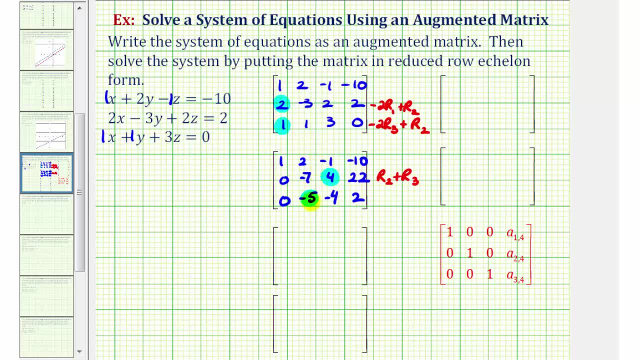 so we don't lose the zero in column one, And since the least common multiple of five and seven is thirty-five, we could obtain a zero in this position if we replace row three with negative five times row two plus seven times row three. So again, the first row is going to stay the same for right now. 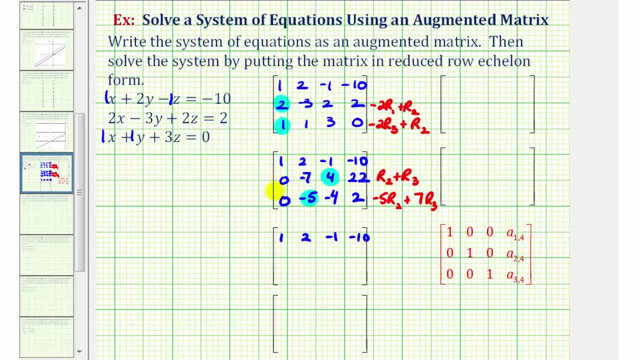 And now for row two, we'll have row two plus row three. So we have zero Negative seven plus negative five is negative twelve. Four plus negative four is zero. Twenty-two plus two is twenty-four. And now for row three, we'll have negative five times row two plus seven times row three. 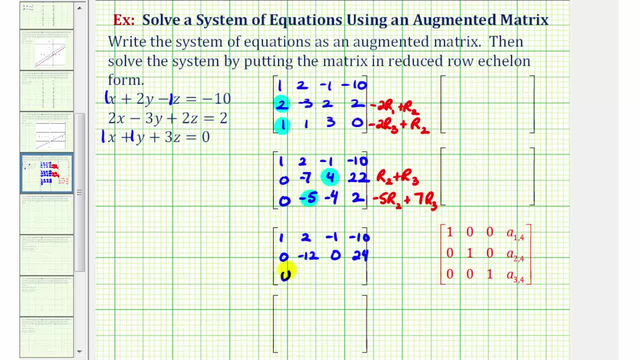 So we have negative five times zero, plus seven times zero, It's still zero. And then we have negative five times negative seven, That's thirty-five, Plus seven times negative five or plus negative thirty-five, That's zero. And then we have negative five times four, That's negative twenty. 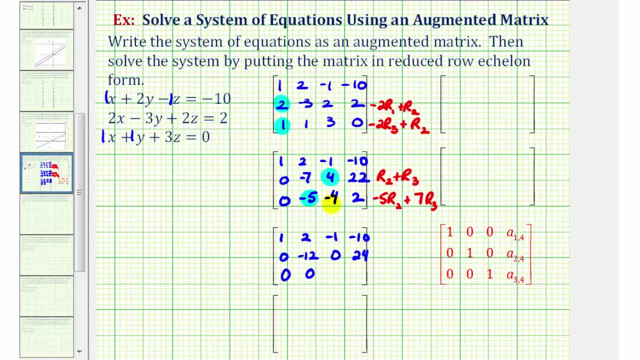 plus seven times negative four, that's negative twenty-eight. so we have negative forty-eight, And then we have negative five times twenty-two, that's negative. one hundred ten plus seven times two or plus fourteen, that's negative ninety-six. 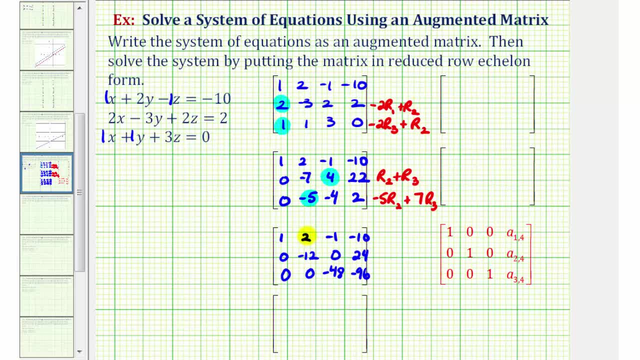 Now, if we take a look at row one, let's obtain a zero in this position here. Let's go ahead and use row two. The least common multiple of two and twelve is twelve, So let's replace row one with six times row one. 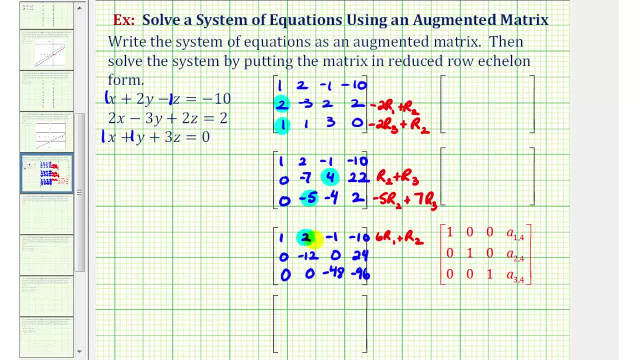 plus row two. We also want the first element in each row to be positive one. So, looking at row two, let's make this negative twelve positive one by multiplying row two by negative one. twelfth. And to make this negative forty-eight positive one, let's replace row three with negative one over forty-eight. 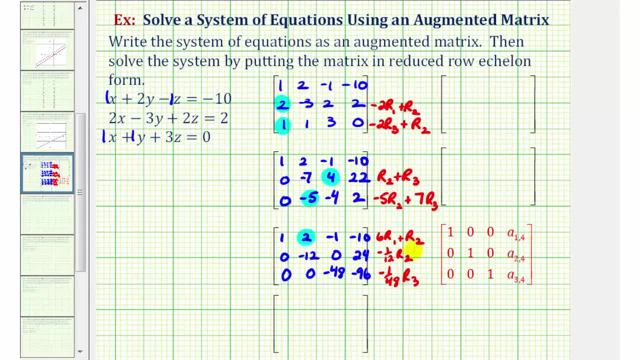 times row three. So let's be careful. here We have six times row one plus row two. Six times one plus zero is six. Six times two plus negative twelve is zero. Six times negative. one plus zero is negative six. 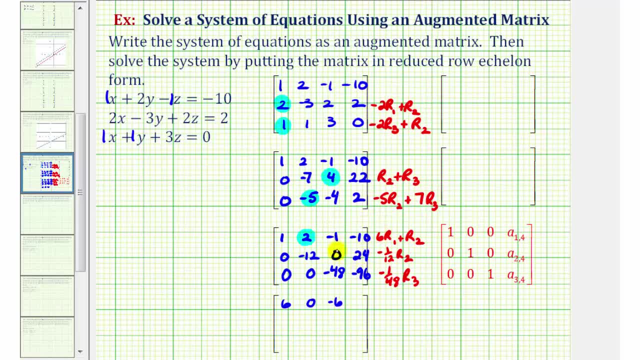 Six times negative. ten is negative. sixty plus twenty-four is negative thirty-six. And now, multiplying by negative one, twelfth is the same as dividing by negative twelve. So we would have zero one, zero negative two. For row three, we would have: 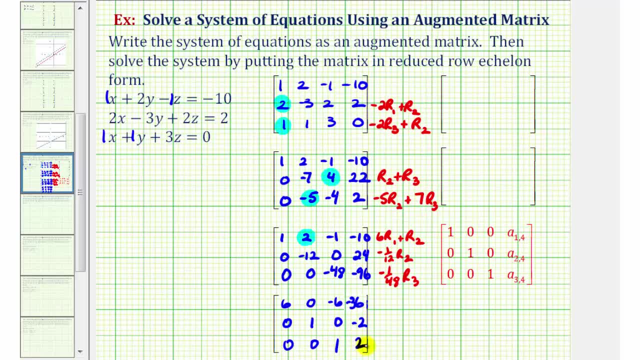 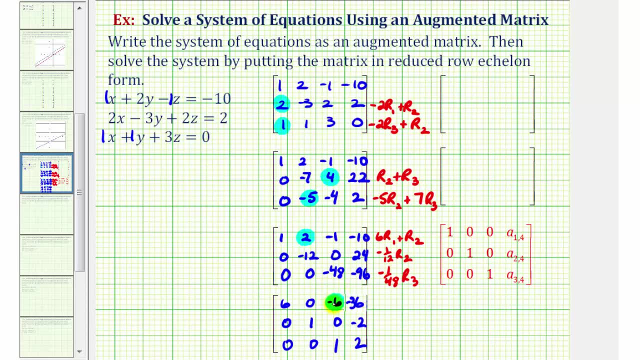 zero, zero one and positive two, And we're almost in reduced row echelon form. We need this element to be zero, So let's go ahead and replace this with six times row three plus row one, So the second and third rows will stay the same. 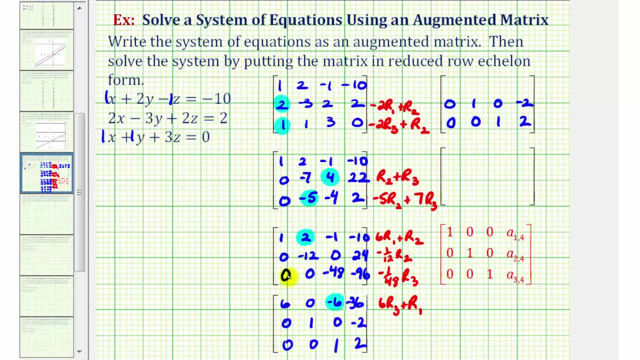 So for row one we'll have six times zero plus six, that's still six. Six times zero plus zero is still zero, And six times one is six plus negative six, that's zero. And we have six times two, that's twelve plus negative thirty-six. 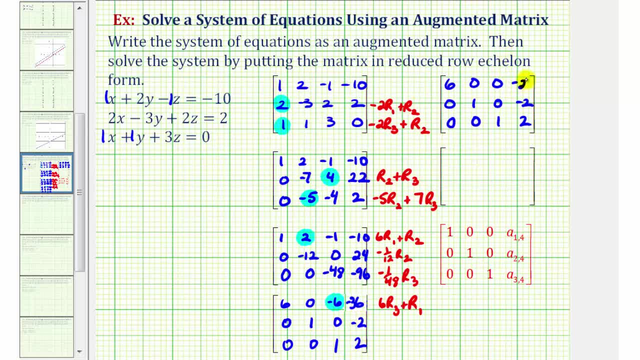 that's negative twenty-four. And now for the last step. we need this six to be a positive one. So we're going to replace row one with one-sixth times row one. So we'll have one zero, zero, negative four, zero, one, zero. 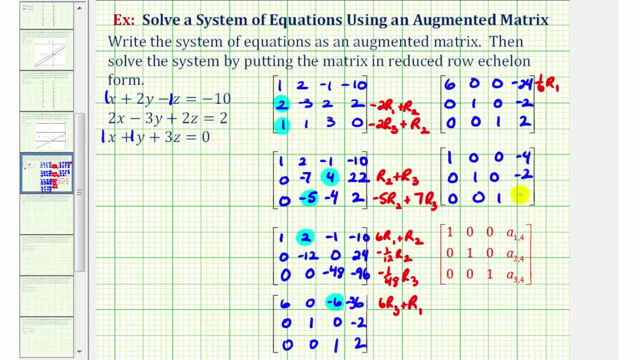 negative two and zero zero one two. Now our matrix is in reduced row echelon form, So if we write this back as a system of equations, we'll have our solution. Remember, these columns represent the coefficients of x, y and z. So row one is telling us that. 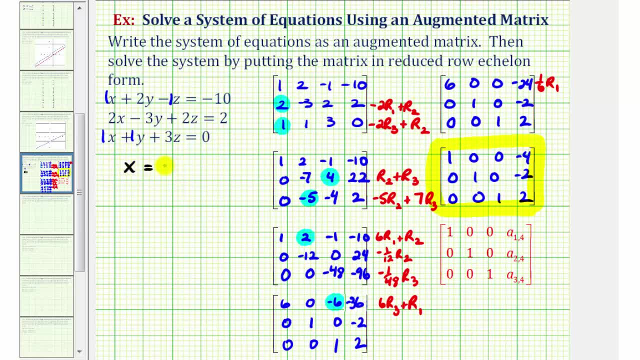 x is equal to negative four. The second row is telling us y is equal to negative two And the third row is telling us that z is equal to positive two. If we want, we can write this as an ordered triple: negative four comma. negative two, comma two. Either way, our system has one solution.